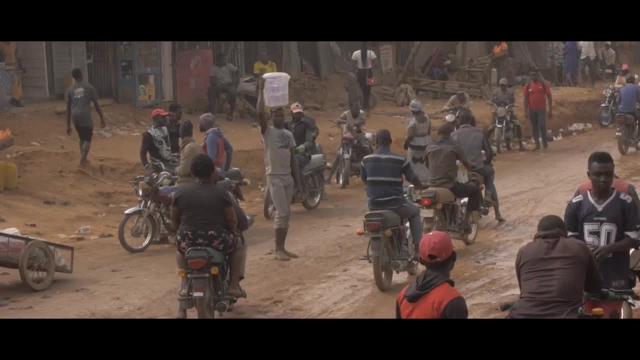 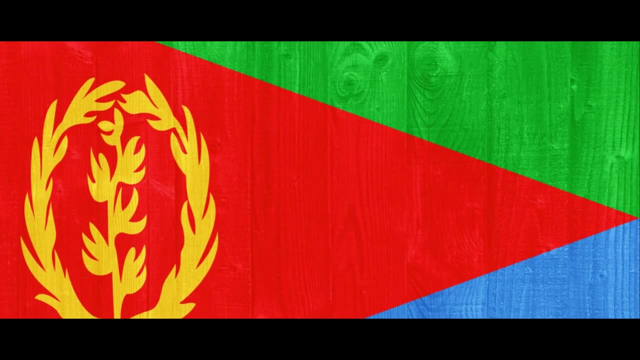 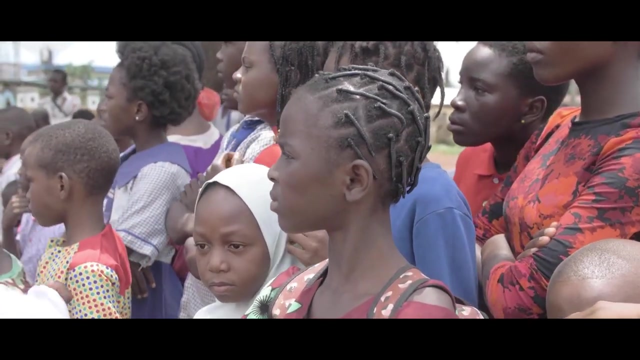 The country's infrastructure, health and education sectors are particularly problematic, all of which contribute to its low productivity. A third measure we can look at is the Human Development Index, or HDI. This index ranks countries based on three key aspects: Life expectancy, education and per capita income. The latest data shows Eritrea near the 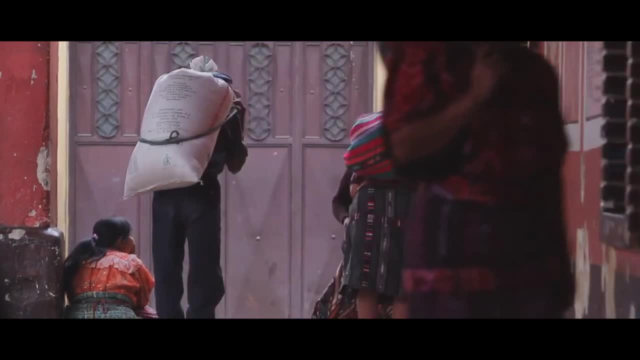 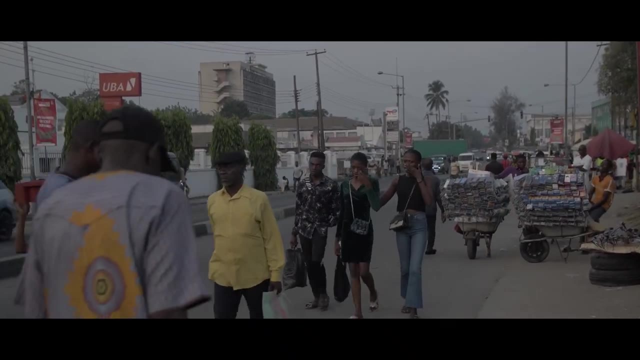 bottom of this index as well, indicating that its population faces significant challenges in health, education and living standards. Each of these indices tells a story, a narrative of economic struggle and stagnation. They highlight how challenging it is to run a business. 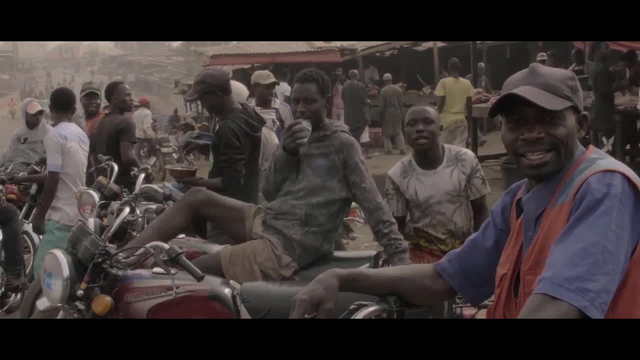 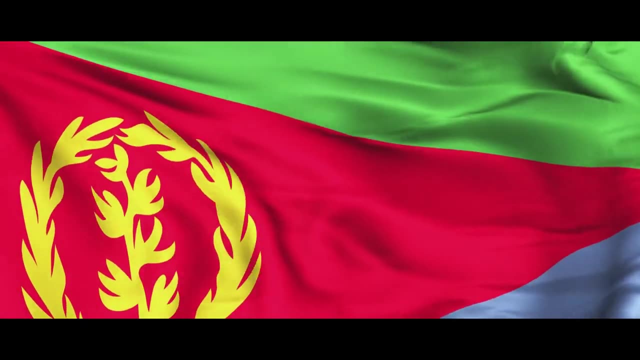 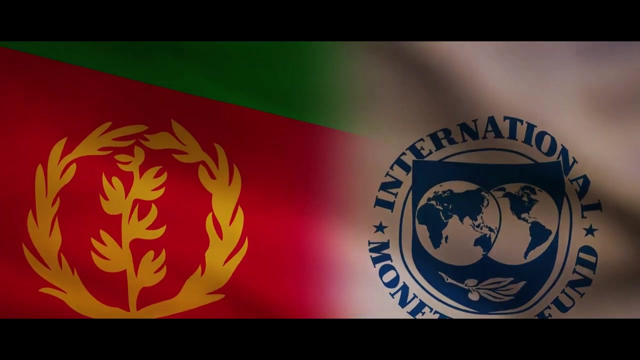 to compete on a global scale and for the average citizen to merely survive. You might wonder: how did Eritrea get here? What factors have led to this bleak economic situation? Well, the answers lie in a complex web of internal challenges and global pressures. Issues like lack of economic reforms. 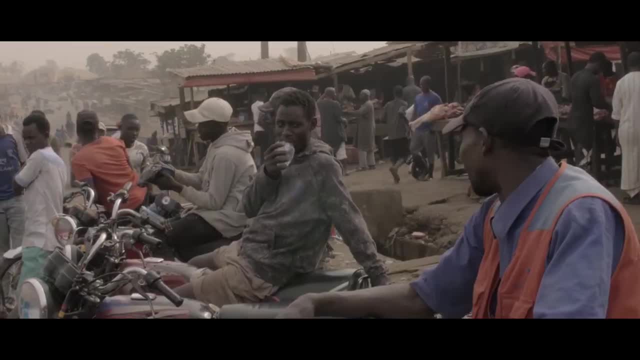 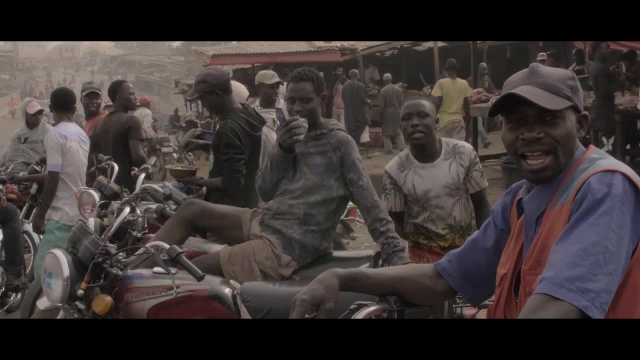 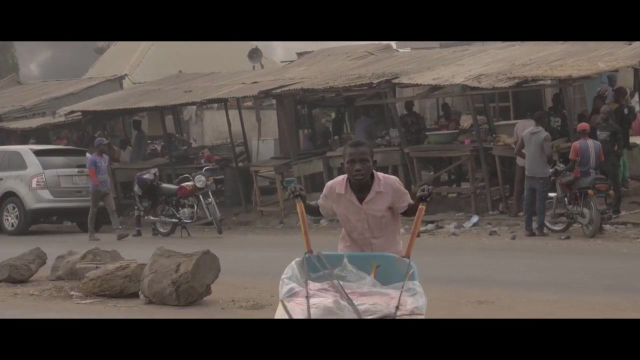 international isolation and a rigid political environment have all played their part. But remember, these numbers are not simply abstract statistics. They represent the lived reality of the Eritrean people. Every low-ranking and negative indicator is a reflection of the hardships faced by individuals and families throughout the country. 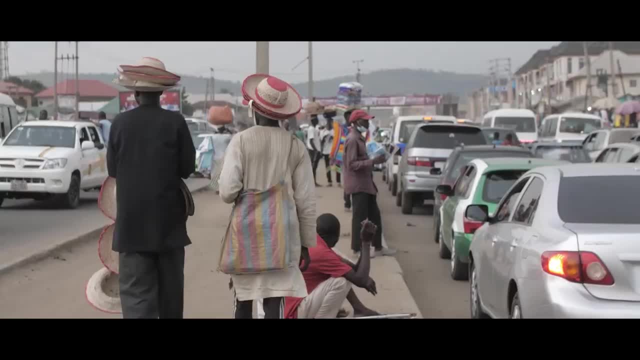 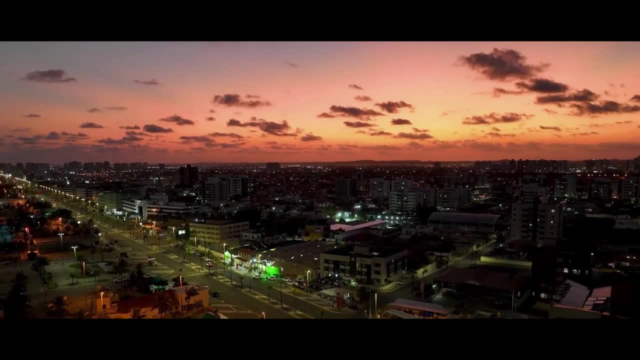 Numbers paint a grim picture, don't they? But what's behind these statistics? Stay tuned as we peel back the layers to understand the forces driving Eritrea's economic woes. Eritrea's economic woes are not due to a single factor, but a combination of several challenges. 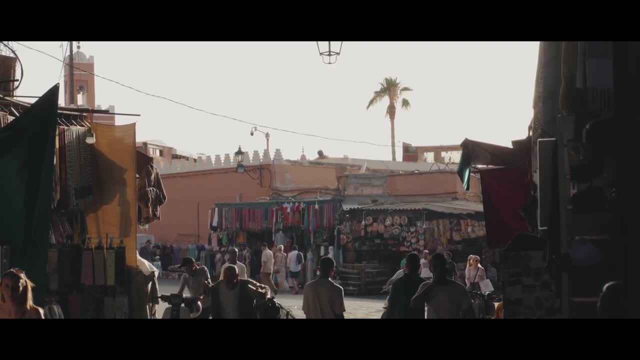 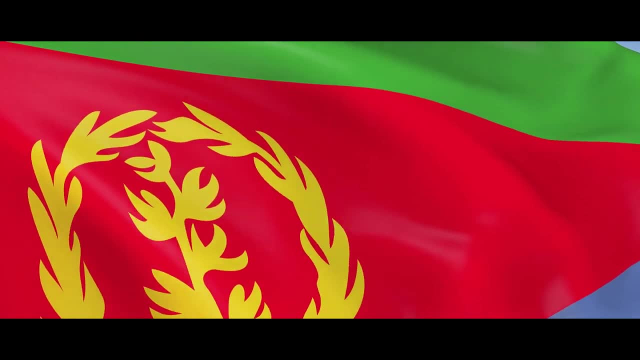 Let's break it down and delve into the main obstacles that Eritrea's economy is currently grappling with. First up is political instability. Eritrea has been marred by years of conflict and tension, both internally and with neighboring countries. This persistent instability- 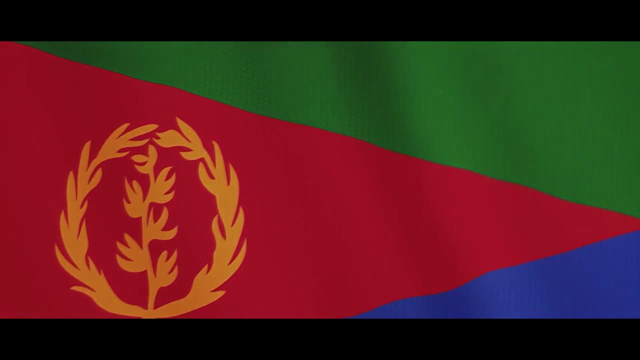 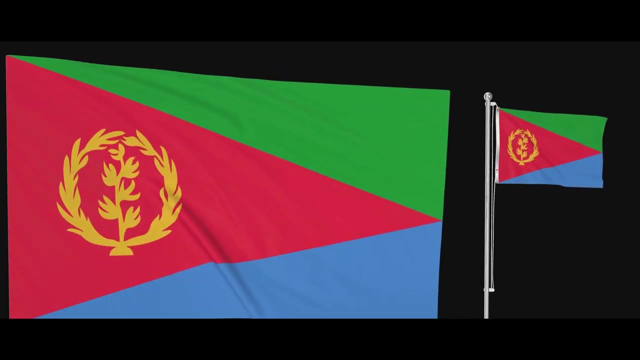 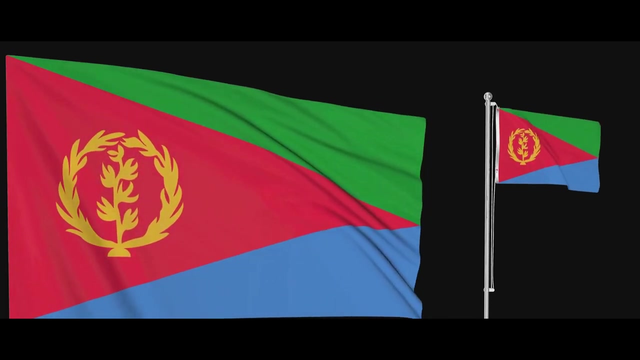 acts as a deterrent for both local entrepreneurship and foreign investment. Investors, both domestic and international, tend to favor stable environments where their investments are secure. The volatile political climate in Eritrea therefore poses a significant hurdle to economic growth. Next we have the issue of foreign investment, or rather the lack thereof. 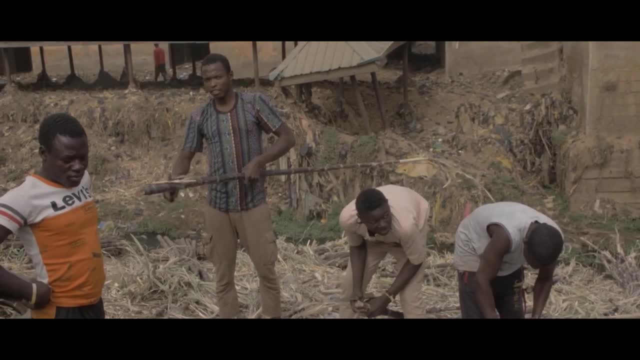 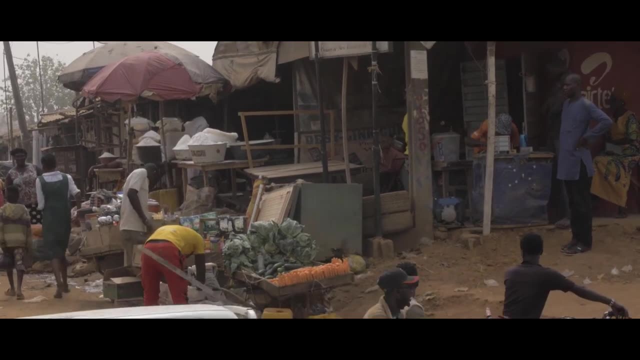 Despite having a wealth of natural resources, Eritrea has struggled to attract foreign investors. This is due in part to the country's restrictive economic policies and lack of transparency. Without foreign investment, Eritrea's economy is missing out on an essential 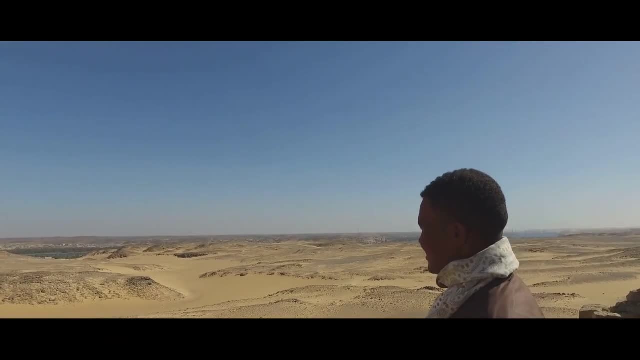 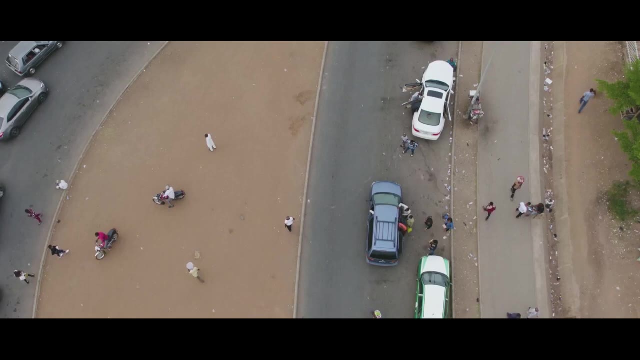 catalyst for growth and development. Then there's the challenge of infrastructure. Eritrea's infrastructure is, to put it mildly, underdeveloped. From roads and railways to power and water systems, the country's infrastructure is in desperate need of modernization. 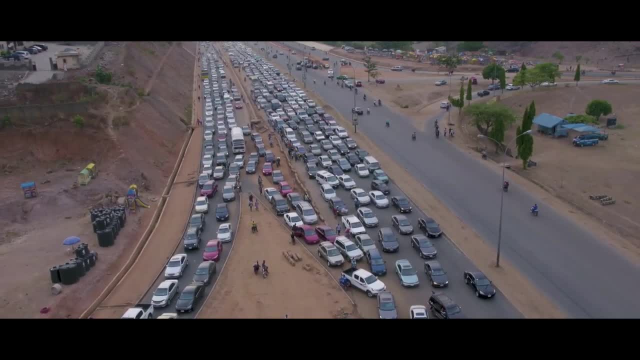 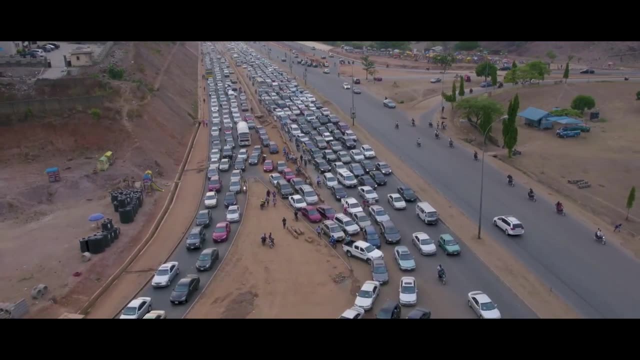 This lack of infrastructure not only hampers economic activities, but also impedes the delivery of basic services, further exacerbating the country's economic struggles. Lastly, there's an over-reliance on agriculture. Agriculture is the backbone of Eritrea's economy. 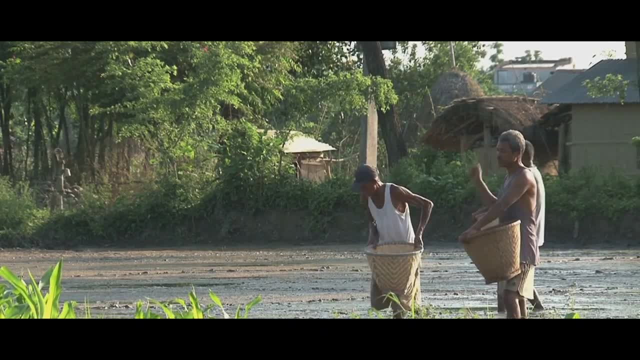 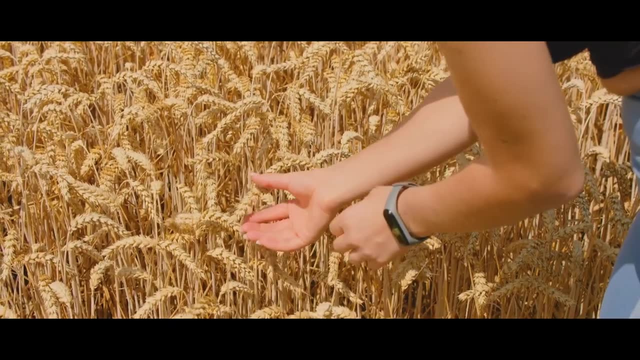 employing a majority of its workforce. However, the country's agricultural sector is plagued by inefficiencies and is heavily dependent on erratic weather patterns. This over-reliance on a single volatile sector leaves the economy vulnerable to shocks such as droughts and floods. 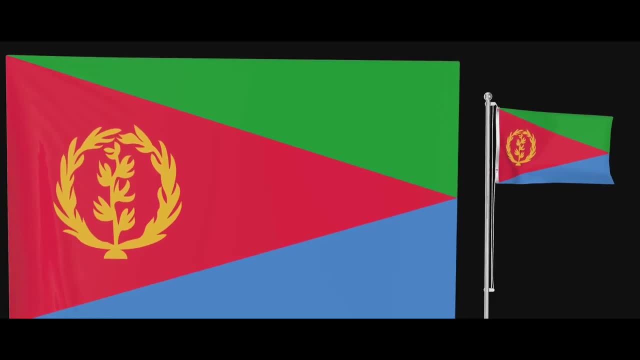 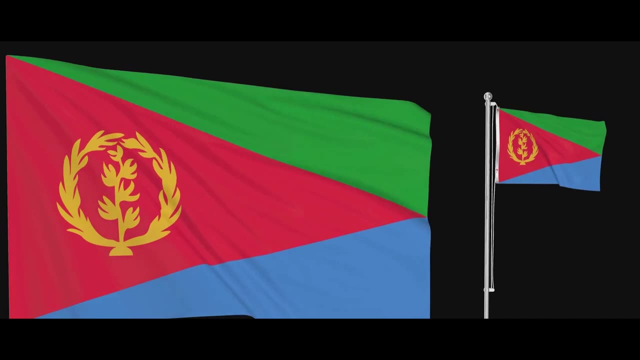 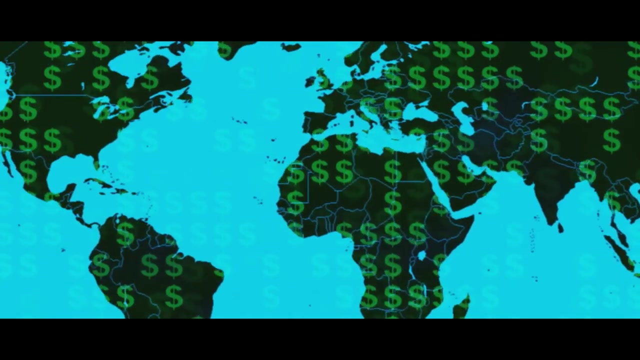 Now let's not forget the role of data and statistics in painting this economic picture. According to the World Bank, Eritrea's Gross Domestic Product, or GDP, has been on a downward trend for the past several years. The country also ranks low on the Ease of Doing Business Index, a testament to the 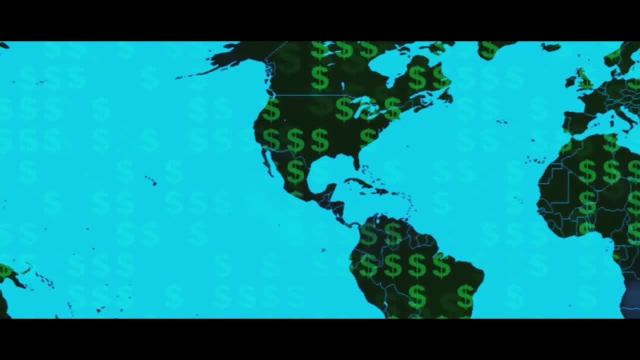 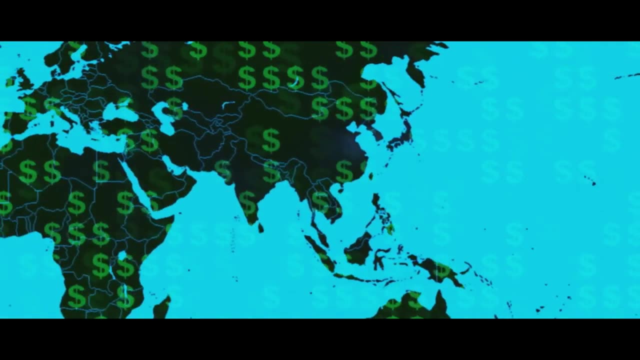 challenges that businesses face in the country. Furthermore, Eritrea's infrastructure score, as per the Global Competitiveness Report, is well below the global average, highlighting the country's infrastructural deficits. But it's not all doom and gloom. 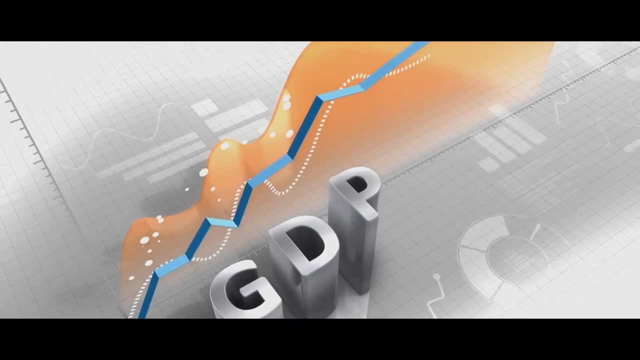 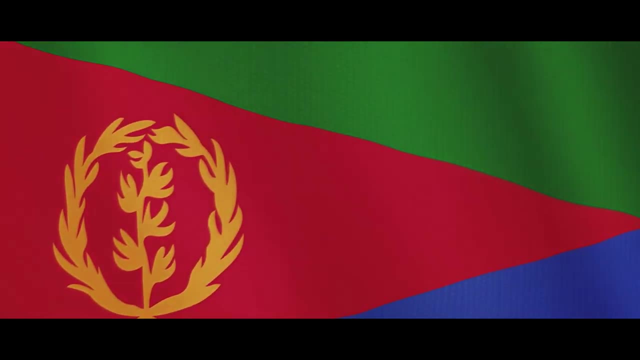 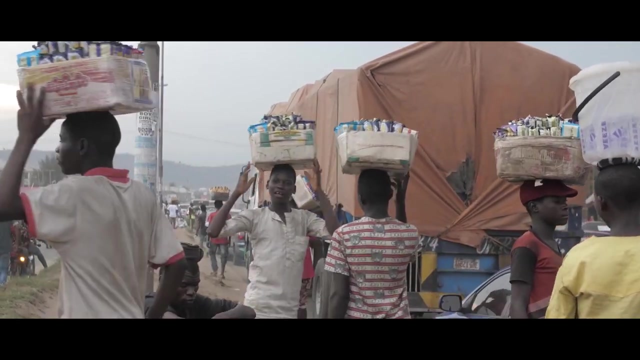 Despite these challenges, Eritrea has a number of assets that could, in theory, fuel economic growth. From its strategic location along the Red Sea to its rich natural resources, Eritrea has the potential to turn its economic fortunes around. These challenges are formidable, but they're not insurmountable. So what's stopping Eritrea? 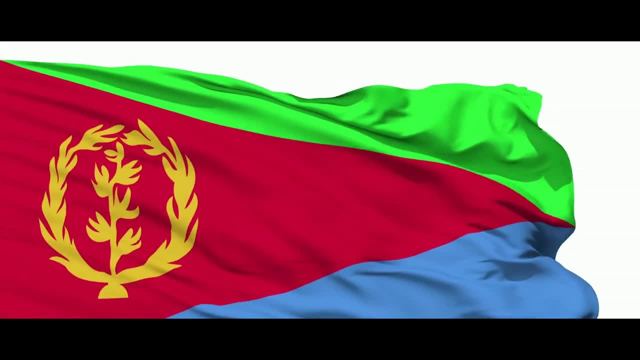 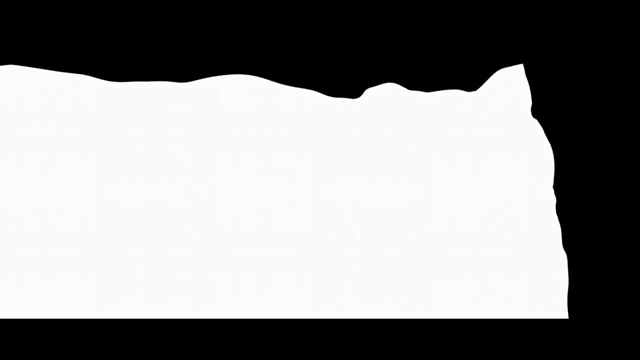 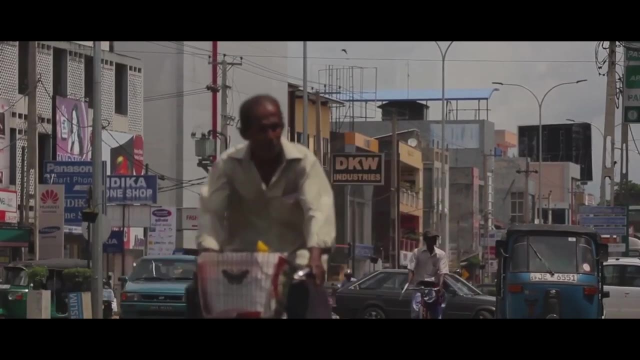 from overcoming them. This question leads us to our next scene, where we'll explore the lack of economic reforms and international isolation that have further compounded Eritrea's economic woes. Stay tuned. Eritrea's economic story is one of missed opportunities and stagnation. The country 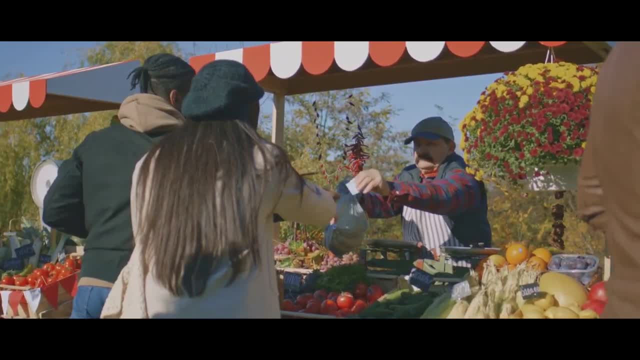 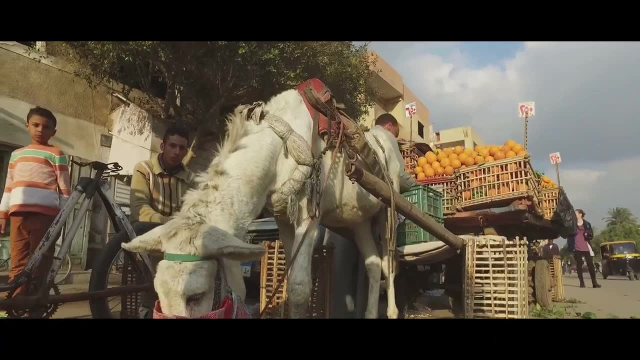 has been slow to implement economic reforms, often choosing to double down on failed policies rather than exploring innovative solutions. This sluggish pace of reform has in many ways hampered the country's economic growth and development. For instance, Eritrea has been 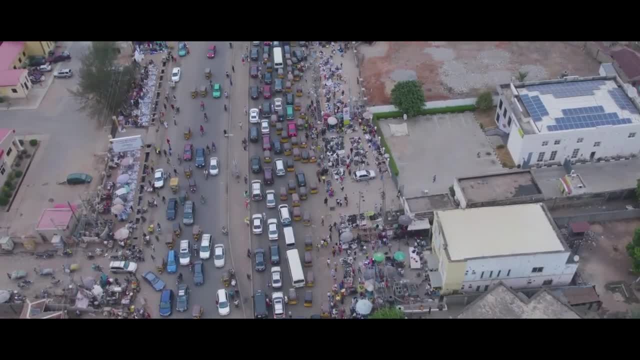 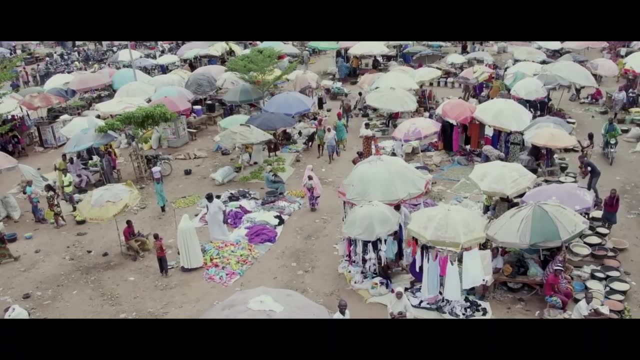 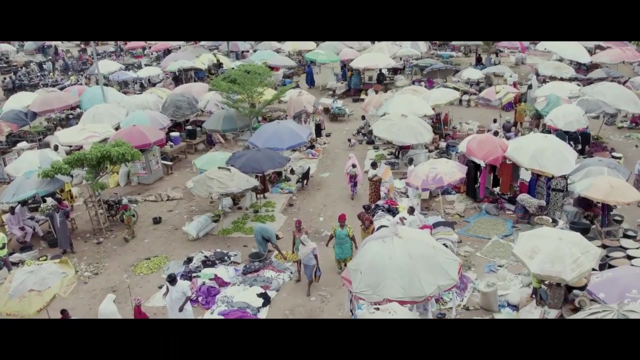 reluctant to liberalize its economy, clinging to a state-led economic model that has proven to be effective in spurring sustainable growth. The government maintains a tight grip on major sectors of the economy, including mining, construction and telecommunications, leaving little room for private sector development. Moreover, the country's 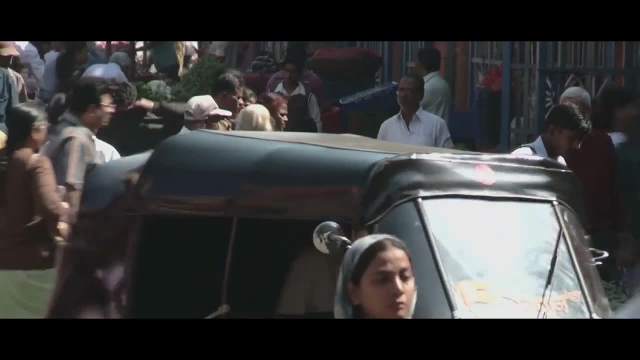 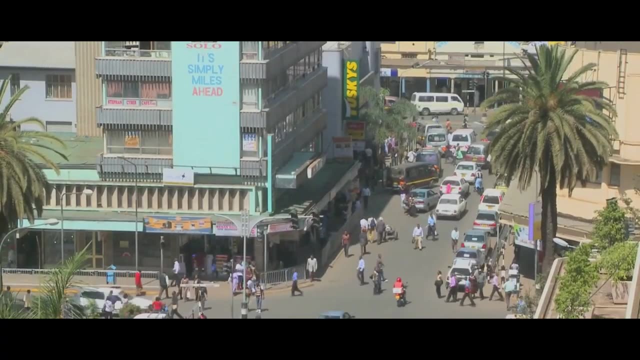 isolation from international markets has greatly undermined its economic potential. Eritrea is largely cut off from the global economy, with limited access to international trade and investment. This isolation is partly self-imposed, as the government has shied away from engaging with the economy. Eritrea's economic growth has been a major challenge for the country. 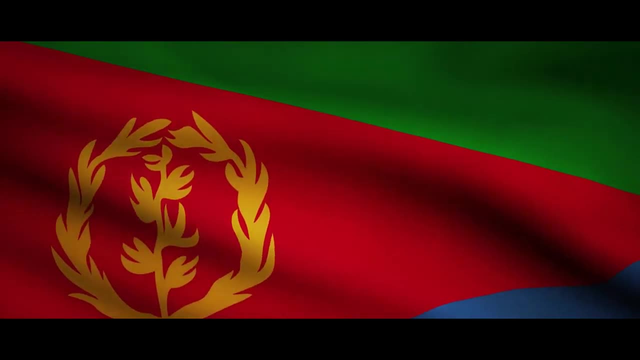 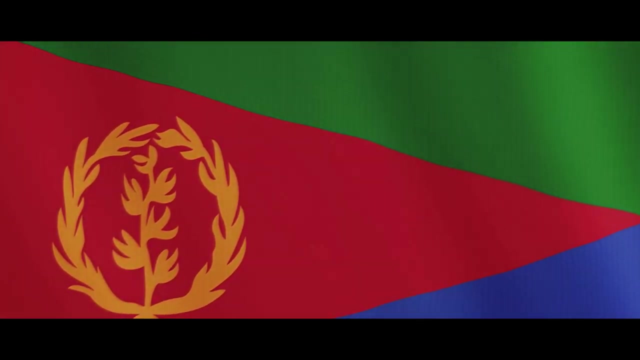 the global economic community. However, it's also a result of international sanctions imposed on the country due to its alleged support for armed groups in the region. These sanctions have further crippled Eritrea's economy, restricting its access to foreign capital and technology. 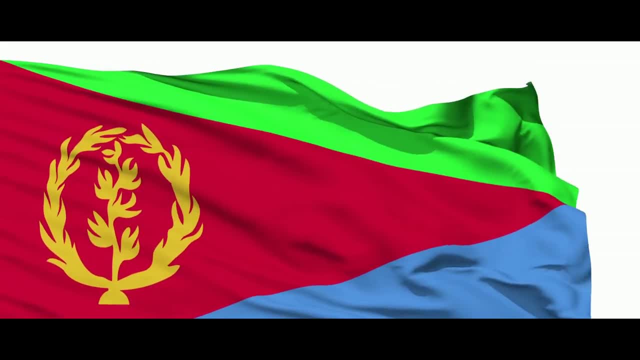 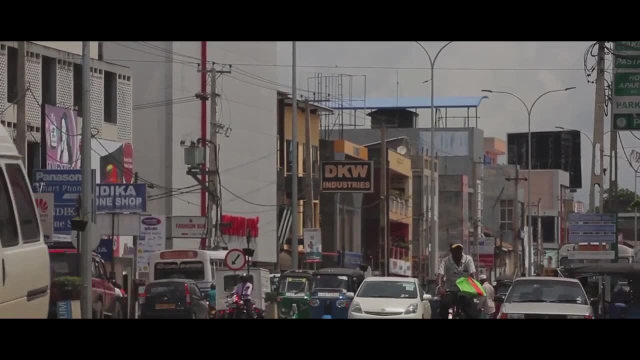 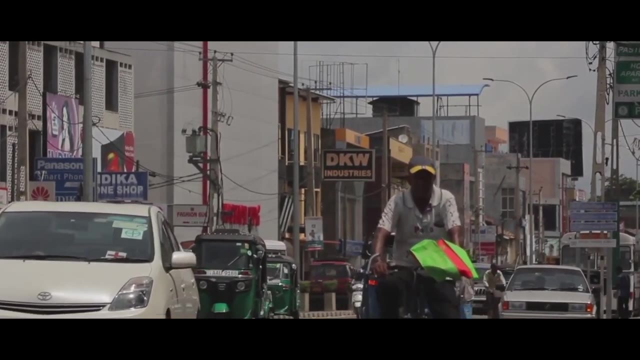 They've also deterred potential investors, who are wary of the risks associated with doing business in a sanctioned country. The impact of these sanctions cannot be overstated: They've not only slowed down the country's economic progress, but also deepened its international isolation, creating a vicious cycle of economic underperformance. 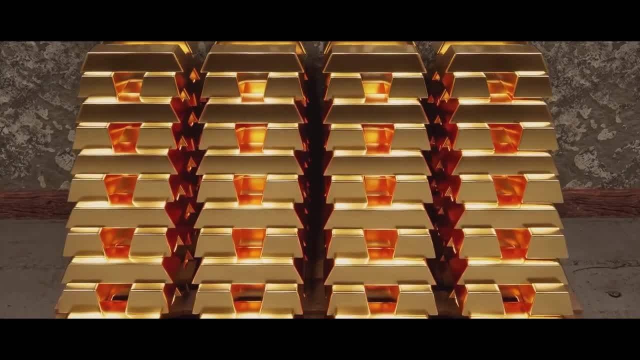 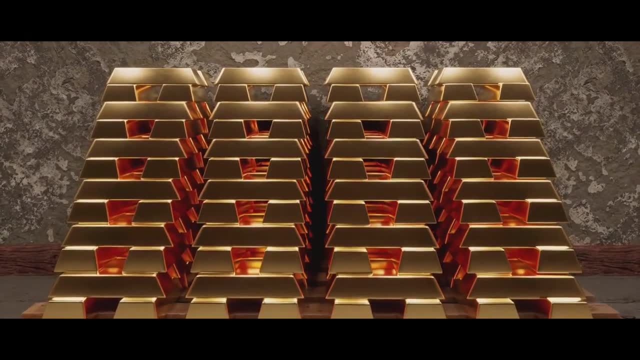 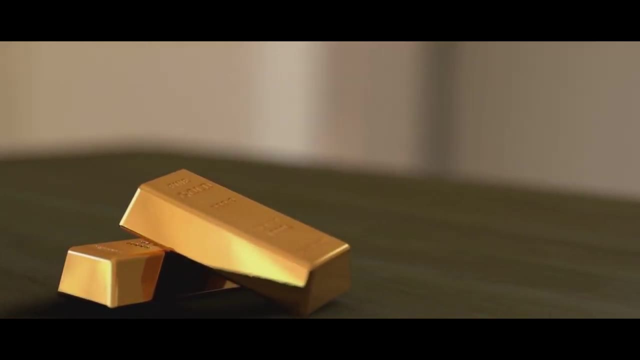 This economic isolation is reflected in the country's poor trade performance. Eritrea's exports are dominated by a single commodity- gold, making the economy highly vulnerable to fluctuations in global gold prices. The lack of economic diversification has further exacerbated the country's economic woes. In conclusion, Eritrea's economic challenges are: 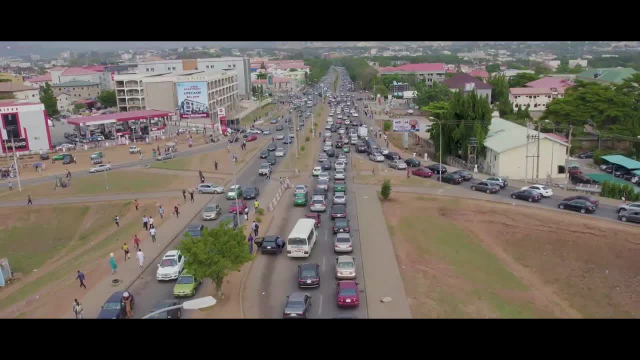 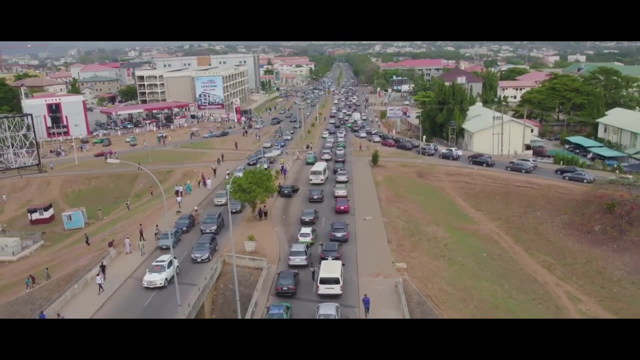 largely self-inflicted, stemming from its slow pace of economic reform and its lack of economic reforms and its isolation from the global economy. The country's reluctance to embrace change and open up to the world has left it stuck in a state of economic stagnation. 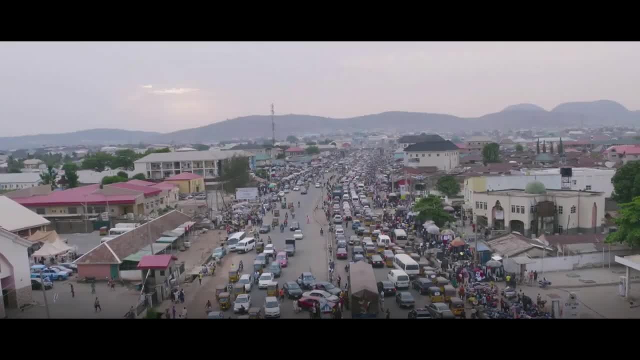 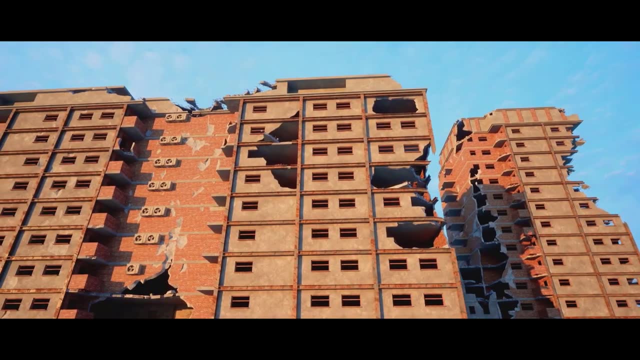 So is there any hope for Eritrea's economy? Eritrea's economy might be the worst in the world, but that doesn't mean it's destined to stay that way. In our journey through the labyrinth of Eritrea's economic landscape, we've unmasked a series of 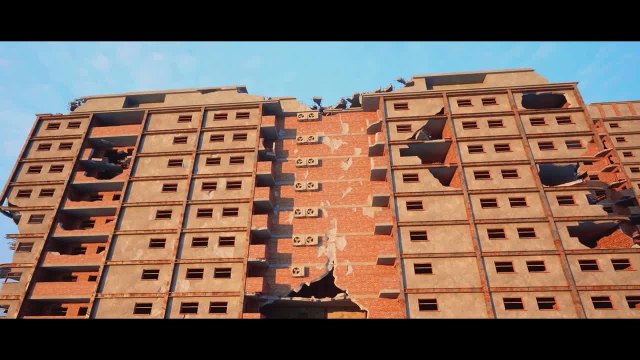 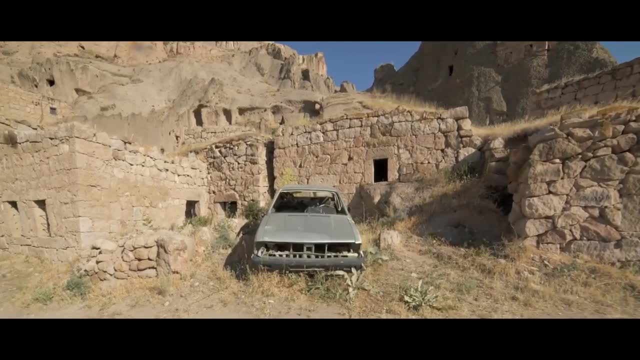 complex challenges, from grim economic indicators to a lack of reforms and international isolation. yet, as we've seen in countless other instances around the globe, no economic situation is ever set in stone. The potential for change and progress is always present, waiting to be harnessed. 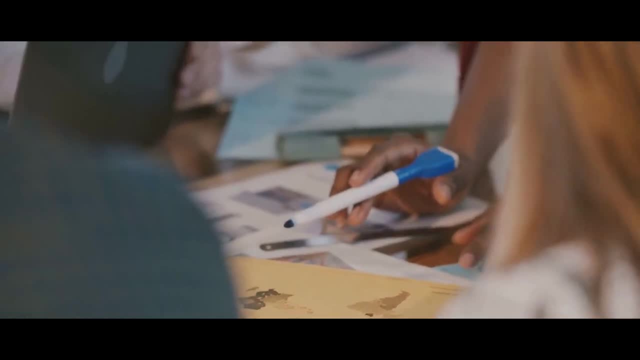 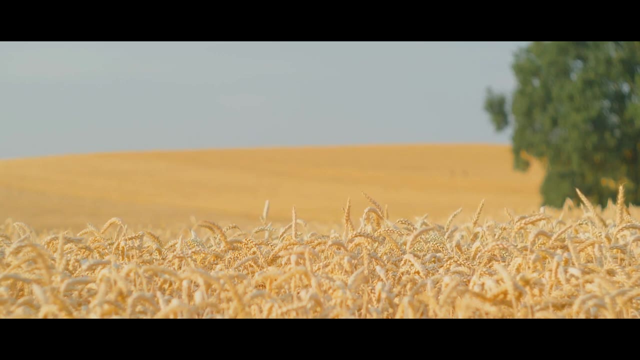 Eritrea's economic woes are not unsolvable. The first step towards a more prosperous future lies in acknowledging the issues at hand. A comprehensive economic reform strategy is needed, one that focuses on diversifying the economy, improving governance and fostering a conducive environment. 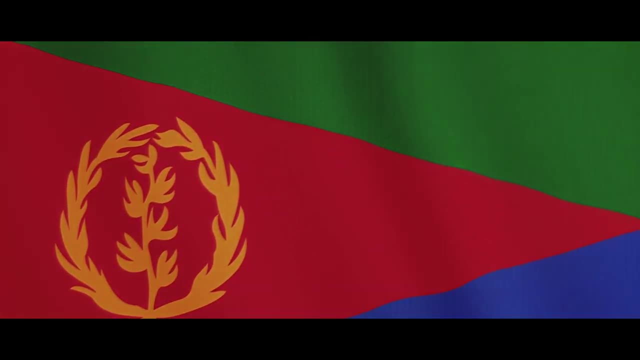 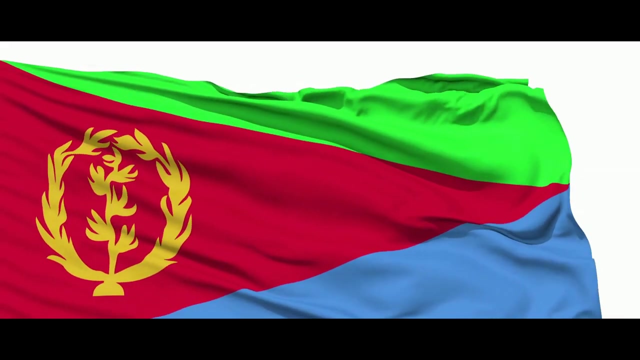 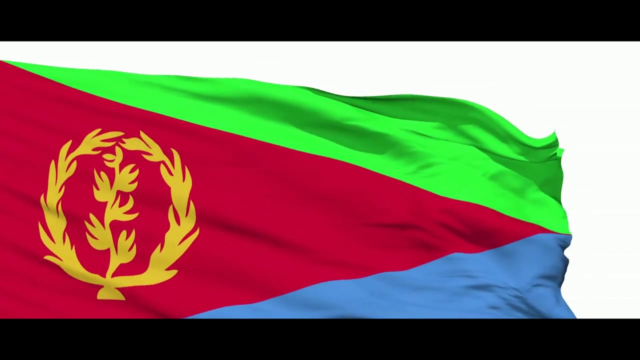 for private sector development. Moreover, Eritrea must work towards mending its international relationships. Global integration is not just a fancy catchphrase. it's a potent tool for economic advancement. By opening its doors to foreign investors and international trade, Eritrea can tap into a 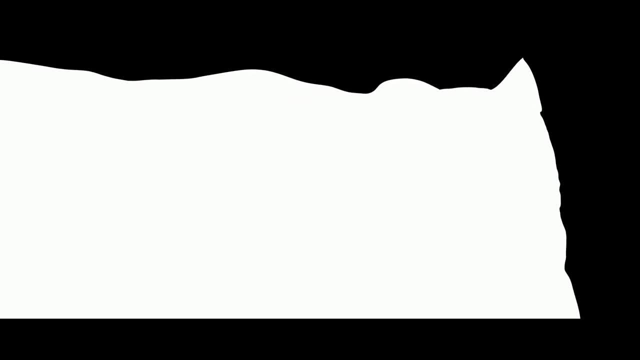 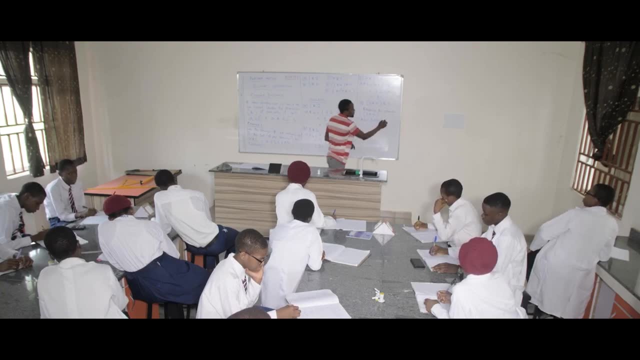 myriad of opportunities that could stimulate economic growth and elevate living standards. Education, too, is a crucial part of this puzzle. By investing in human capital, Eritrea can cultivate a skilled workforce that can drive the development of the economy. Eritrea's economic 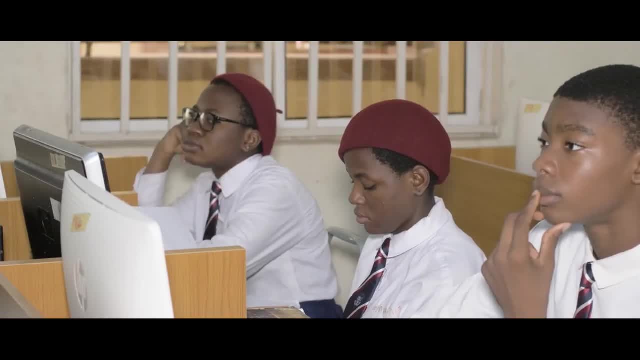 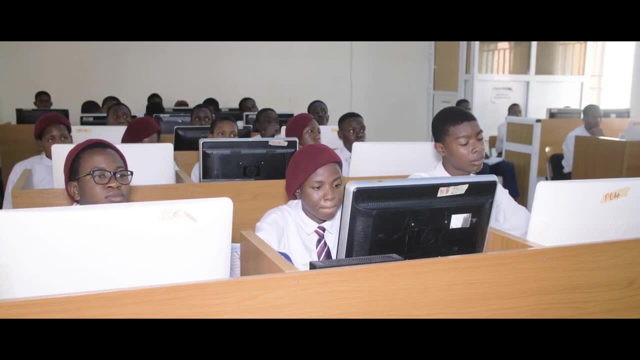 development can drive innovation and productivity. And let's not forget about technology: Embracing the digital revolution can accelerate Eritrea's economic transformation, paving the way for a more connected and prosperous nation. The road to economic recovery will not be easy. 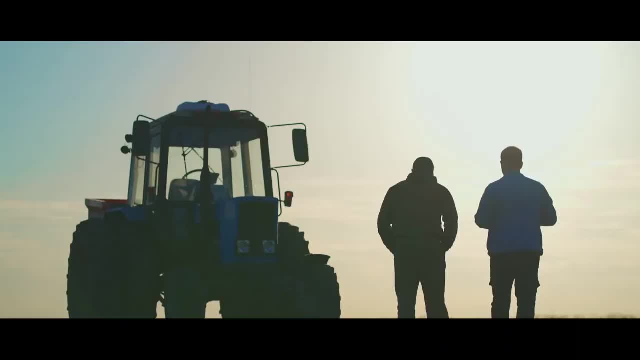 and it will not be quick. It will require sacrifice, perseverance and a commitment to long-term goals. But with the right policies and the collective will of its people, Eritrea can rewrite its economic narrative. We invite you to continue this conversation. Let's. 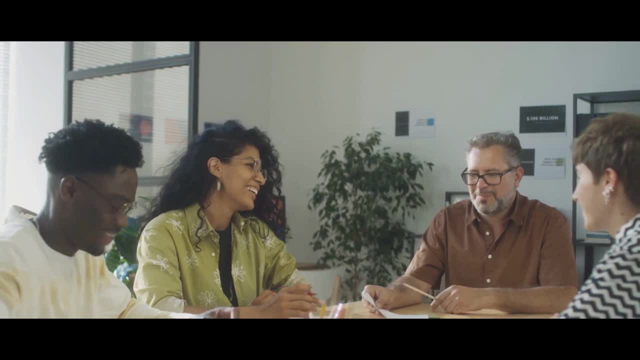 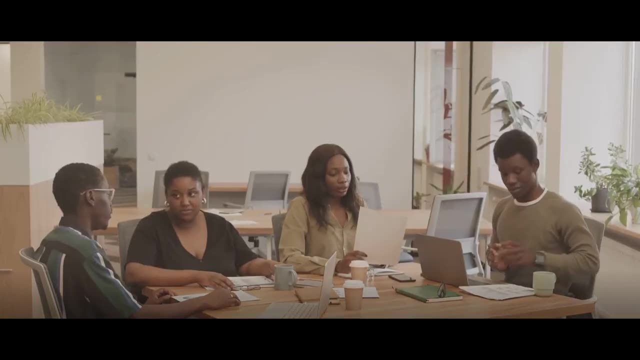 brainstorm together, share ideas and inspire change. Your thoughts and insights can make a difference, So let's create a dialogue that sparks action and fosters hope. Remember, economies can and do change, and Eritrea's is no exception, So don't forget to.